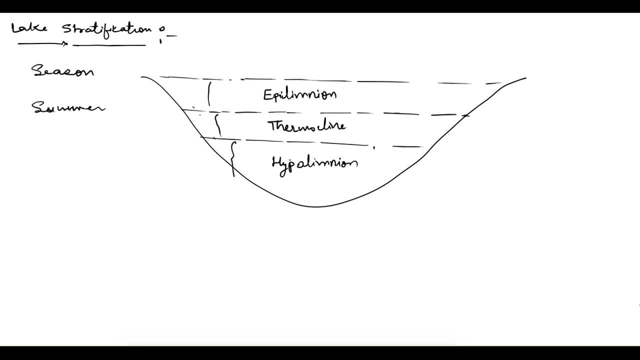 In case of winter it will be different. So in case of summer, these three layers are formed: epilimnion, thermocline and hypolimnion. So epilimnion, let's see these one by one. Epilimnion is your top layer and it has, obviously, if it is on the top, so it is in contact with the air, So it has highest DO and because of this air movement, mixing also takes place. 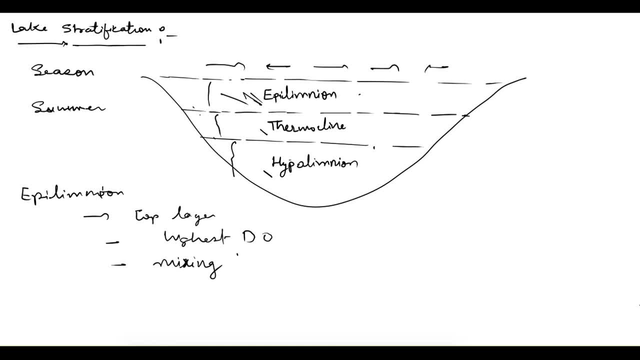 That is, mixing of water in this layer only- I mean intermixing between the layers- cannot take place because of this difference in temperature. For this particular layer, mixing takes place. That is your epilimnion and for the temperature gradient in this zone we can generally say temperature gradient is less than 1 degree Celsius per meter depth of water. 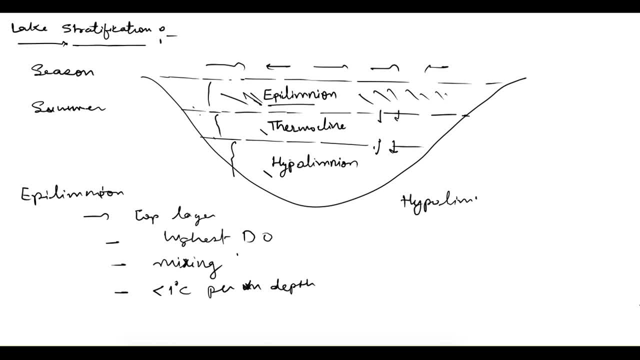 So this layer is your hypolimnion, So it is on the bottom side. So obviously DO is minimum. DO is minimum and in this case some anaerobic activity can happen here and aerobic and temperature gradient also. in this case also, it is less than 1 degree Celsius per meter depth and mixing does not take place in this layer. 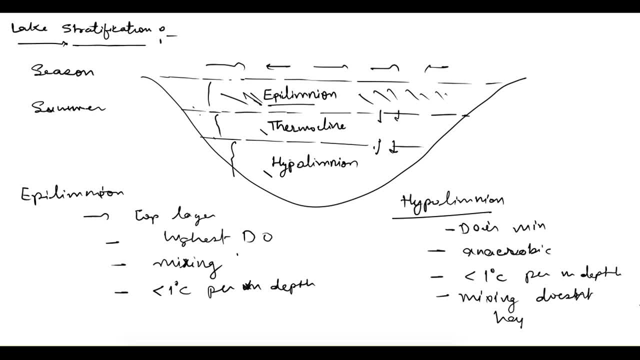 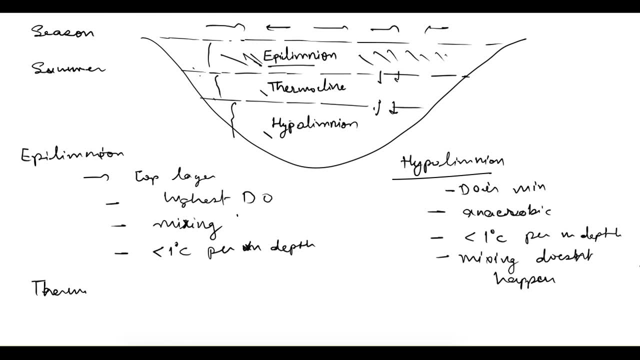 And these two layers are divided by another layer, That is, your thermocline. So thermocline, it is also known as metal imnion, and it has highest temperature gradient, that is greater than 1 degree Celsius per meter depth of water. So all three layers are evenly distributed. but this layer also gives you 5 taste, 7 taste, 7 Hart stay, 8, heat type layer, and so on. 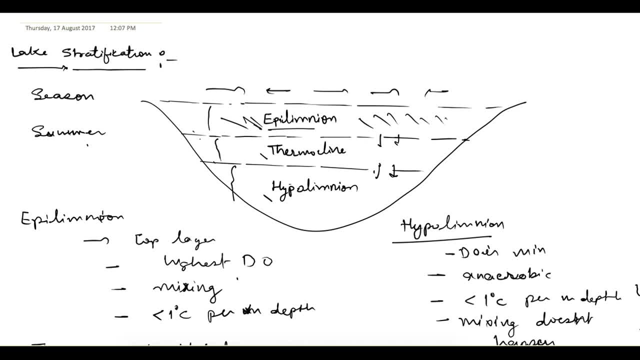 And then what we unlock is that there is onevariable layer in this layer. it is called protodindung layer. So this Buchan layer of onevariables naturally disappear in the. So this kind of layer stratification happens in case of summer, Whereas as the season changes from summer to winter, 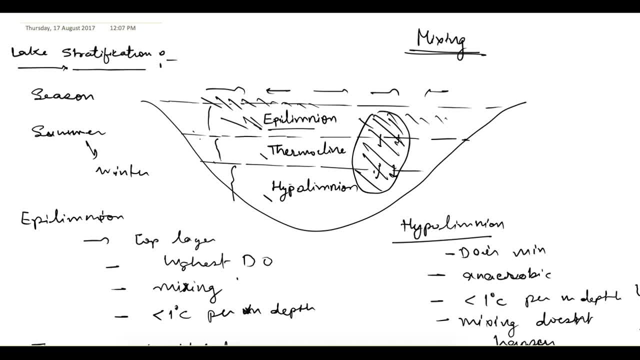 So what will happen? This upper layer, Temp Return of this upper layer will start to decrease. kind of leg stratification happens. in case of Summer layer will be the coolest. so if the temperature is below 4 degrees Celsius, you should know that water has highest density. highest density as I mean. 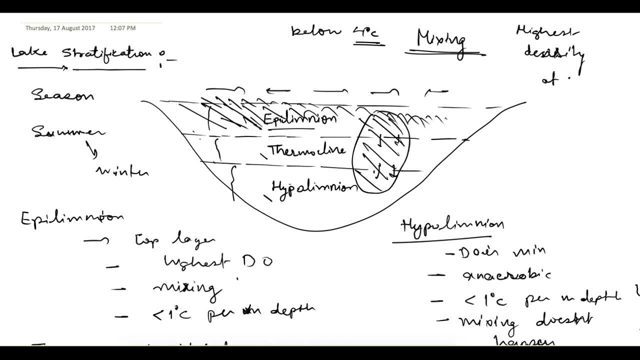 highest density at 4 degrees Celsius, and if the water becomes warmer or cooler than this, then the density decreases. so if this top temperature- I mean top surface temperature- is less than 4 degrees Celsius, or we can say that if the ice formation happens, then this top layer will be cold coolest and it will 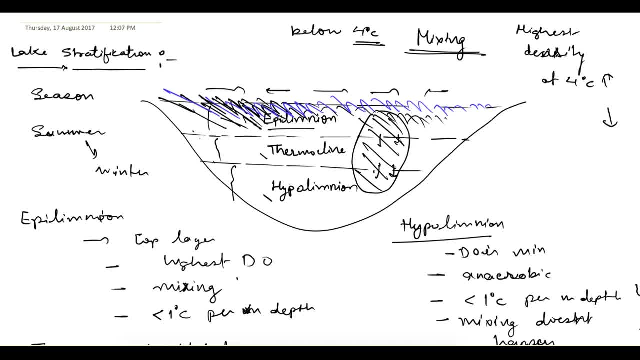 be. I mean, the density will be least here and as we go down the temperature will be more. here the temperature will be more in case of summer and on the top temperature is least. so this happens in case of winter, you and again. if the season changes from winter to summer, summer, there will be a 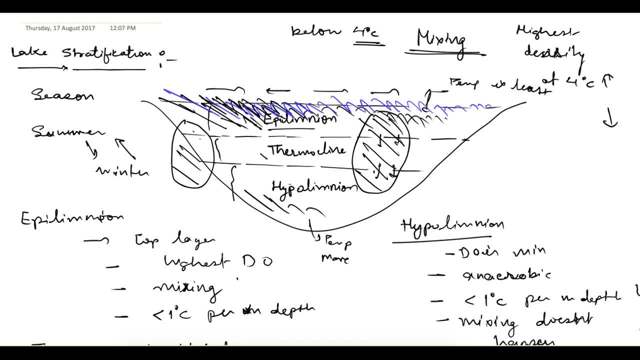 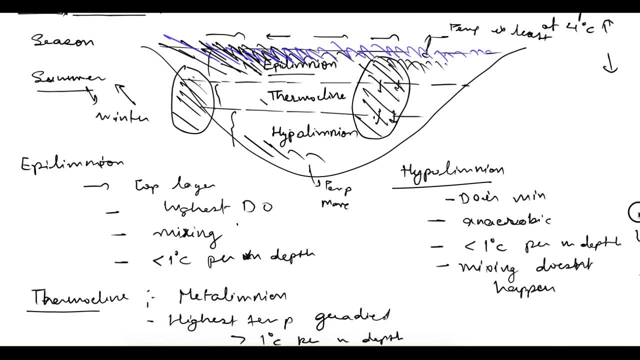 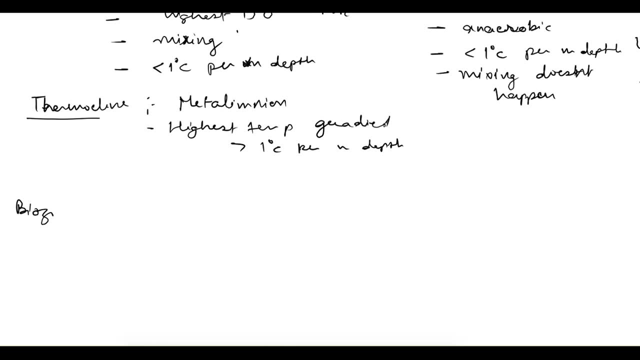 time again, all these three layers will be of same temperature and mixing will take place and in some summer, these again these three layers will form. that is your lake stratification. after that we can see biological zones in lakes- biological. so three zones are formed in case of lakes. that is your euphotic zone: euphotic. 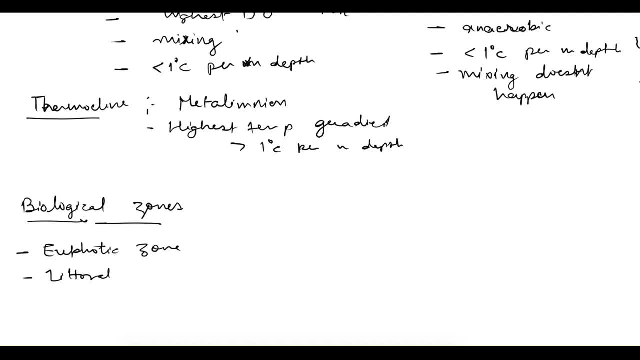 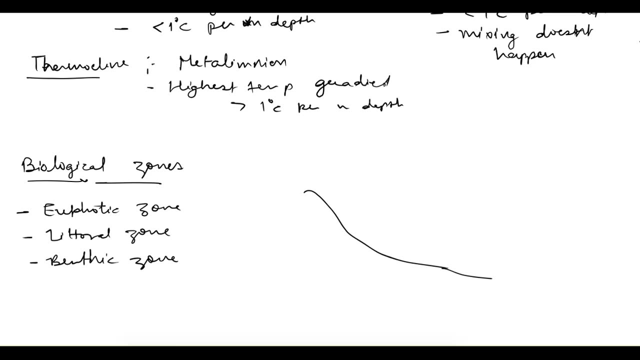 zone and then there is littoral zone and benthic zone. so only you should know where all- all I mean where all- these zones exist. so if we show this is your section of lake, so euphotic zone occurs on the top most side. this is your, I mean. 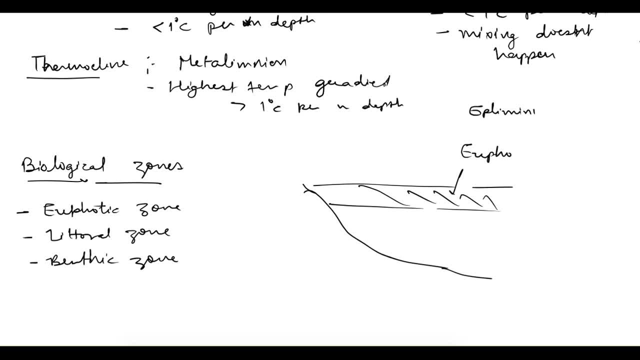 normally it will be in this epilinear layer, but if it is, if the lake is clear, and so how does it? I mean how this euphotic zone is decided. it depends upon whether the sunlight can easily penetrate. if sunlight is entering, I mean up to the depth where★★★★★★★★★★★★★★★★★★★★★★★★★★★★★. BESIDES. HERE WE CAN KEEP THE movement. BESIDENisy NEEDED TWO WIDE HIP LINE IS READY FOR THE SUN. Dっと IT WON'T FEEL quedar lesley. easter spells in leah reed. a 집에 satie might a permanent and this side of the body form, and I am interested in what is loe dell person when this is due and what you want to do is still managers, you can find the meu. 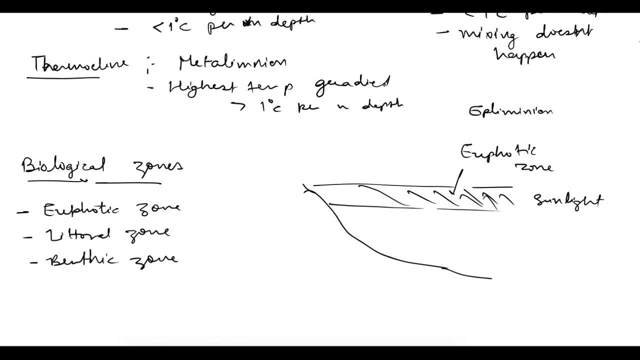 I mean up to the depth where sunlight is entering properly. that will be your euphotic zone. so if lake water is clearer, then up to up to this lowest- that is hypolimnion layer also- euphotic zone can exist, but normally it will be. 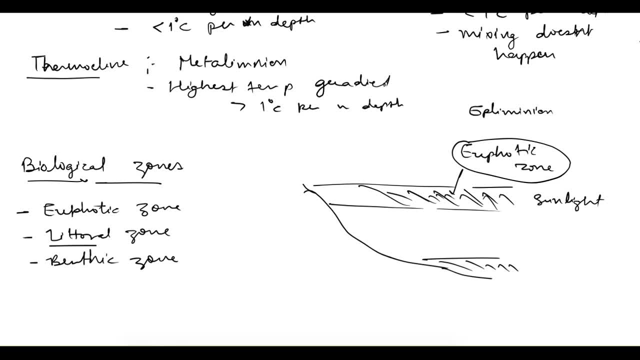 in your epilimnion layer. next is littoral zone. so littoral zone is your these shore kind of zone, I mean on and the bank of this lake, where the, where some plants can exist and plants can grow, that will be your littoral zone and 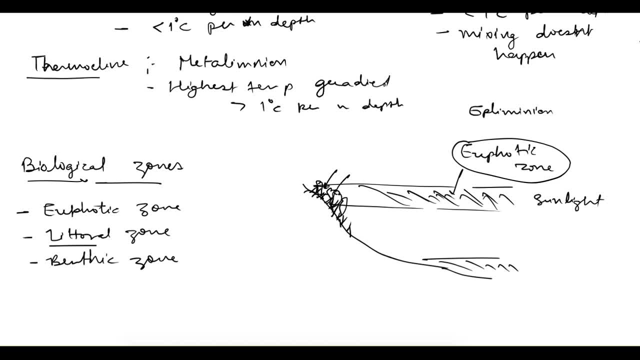 it will be in water but the sunlight is reaching here so photosynthetic photosynthesis can happen and some plants can grow. and benthic zone is your, these muddy zone below the hypolimnion. this is your benthic zone and here is 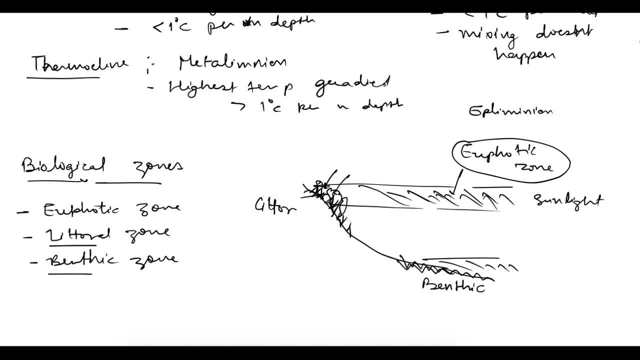 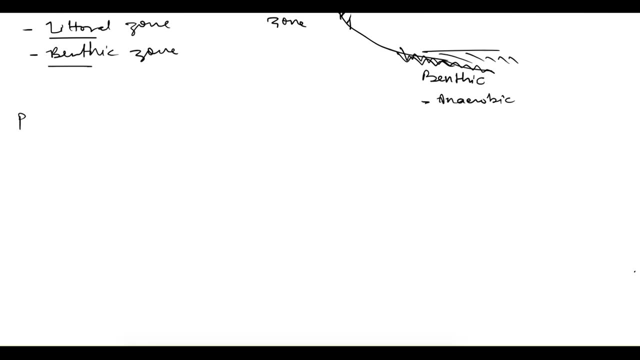 your. this one was your littoral zone, so this will be total in anaerobic condition. these are the three biological zones. after that we can see some little classification of lakes depending upon productivity. that is first. one is your oligotrophic lake. so productivity I mean with the productivity we mean here is if the algae can grow easily or not. 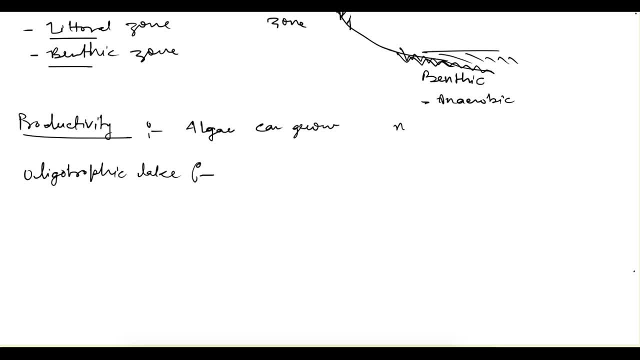 so that depends upon the nutrients present in water. and if we are leaving the waste water in the lakes, if we are discharging the waste water in the lakes, then we are supplying carbon and phosphorus and nitrogen and these are the very good nutrients. these are the very good nutrients. 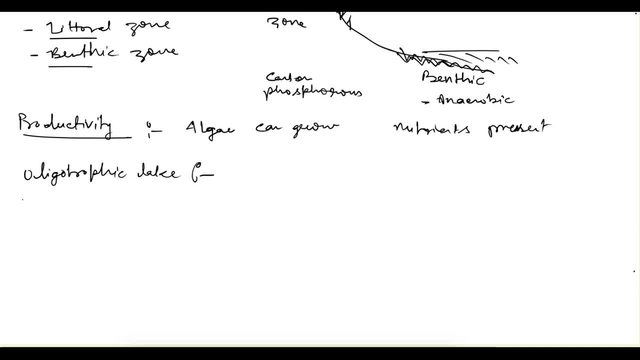 for the growth of these algae and other things. So that is your productivity. So oligotrophic lake has low productivity because it has very limited supply, of limited nutrient supply And in this lake- these are very clear lakes and euphotic zone that we just saw- the different 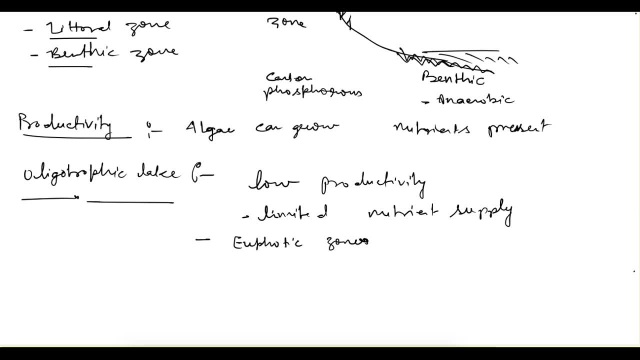 zones and Euphoric zone exists up to high-polymeria. These are very clear lakes we can say: Next one is your Mesotrophic lake. So obviously it is a lake of little more productive than this. so algae can grow- not a lot, but algae can grow here. 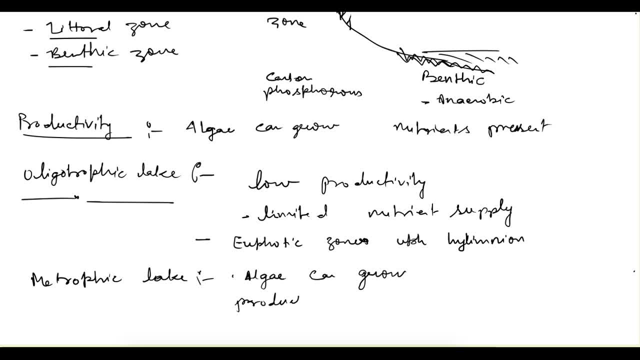 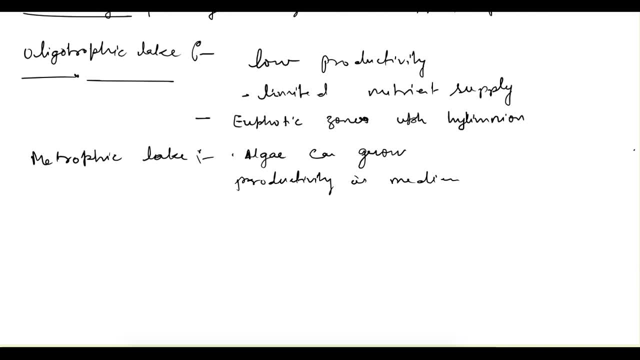 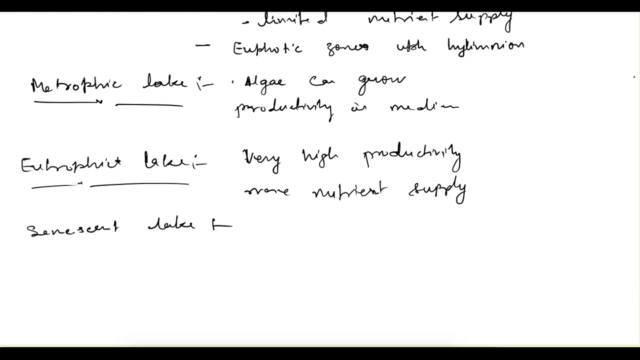 so we can say productivity is medium. then after that you have your eutrophic leg. these have very high productivity. very high productivity that means the nutrient supply is very high, more nutrient supply. and the last one we can say is senescent lake. senescent with the name itself if the meaning is that the lake is very old. 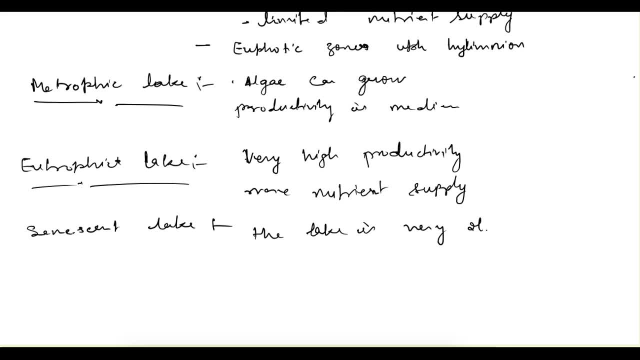 lake is very old and it has been occupied by mostly algae and other marshy vegetables and vegetative plants. so that would be your senescent lake. so one more definition that we can see here is eutrophication of lakes. so eutrophication. 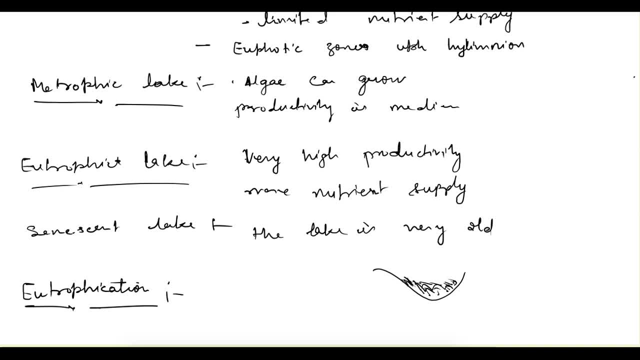 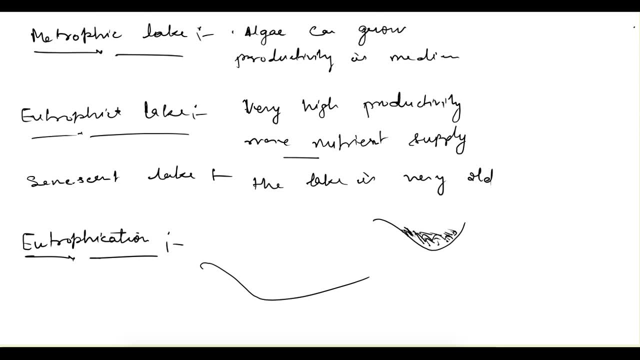 simply, it is related to this eutrophic lake. what we saw: if, if the productivity is high, that means more nutrient supply is there, then with time more algae, algae will grow and most of the lake, i mean this space- will be occupied by algae and not much water will be left in this lake. so this lake will be of.